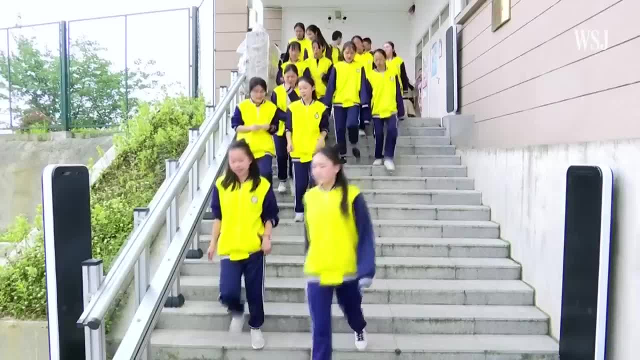 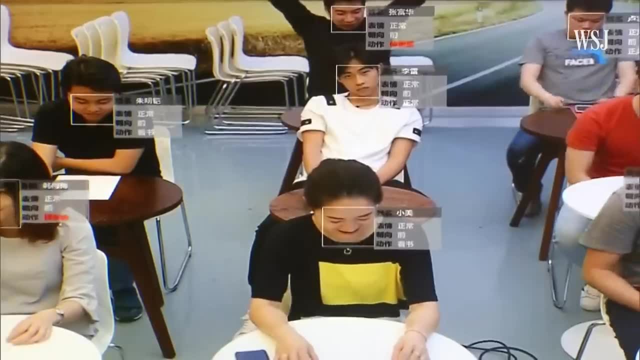 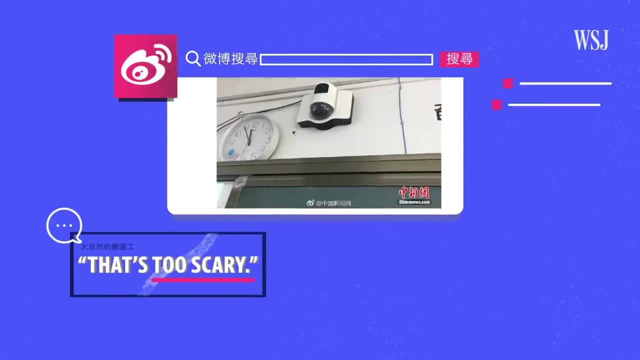 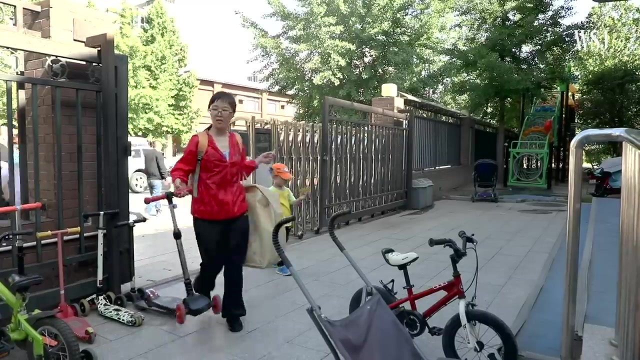 Classrooms have robots that analyze students' health and engagement levels. Students wear uniforms with chips that track their locations. There are even surveillance cameras that monitor how often students check their phones or yawn during classes. These gadgets have alarmed Chinese netizens, But schools say it wasn't hard for them getting parental consent to enroll kids into what. 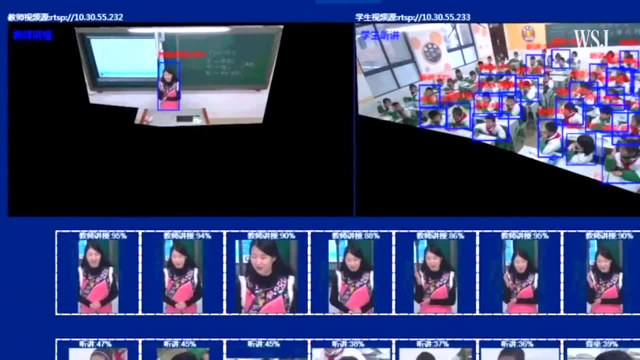 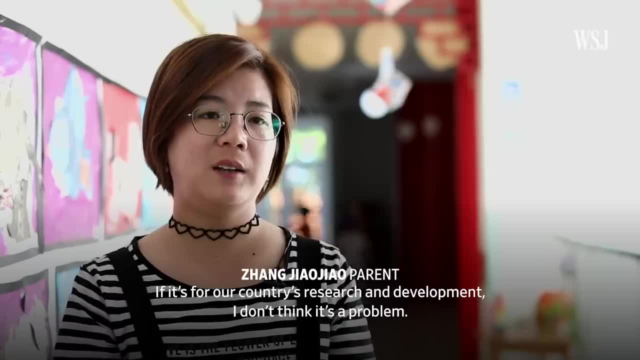 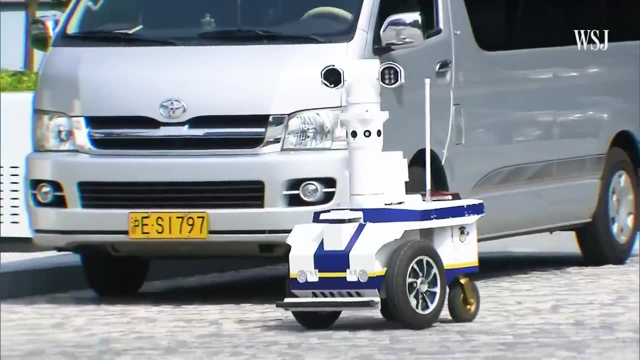 is one of the world's largest experiments in AI education, A program that's supposed to boost students' grades While also feeding powerful algorithms. For the sake of national research and development, I don't think there's a problem. The government has poured billions of dollars into the project, bringing together tech giants. 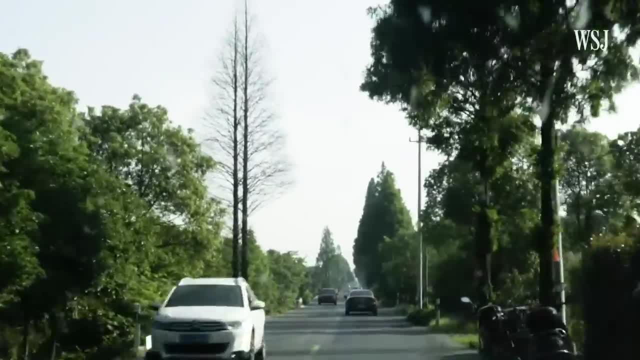 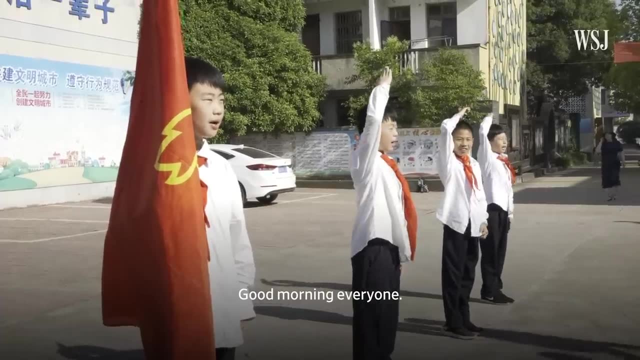 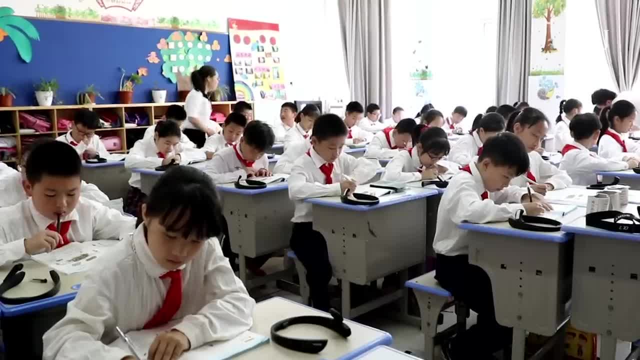 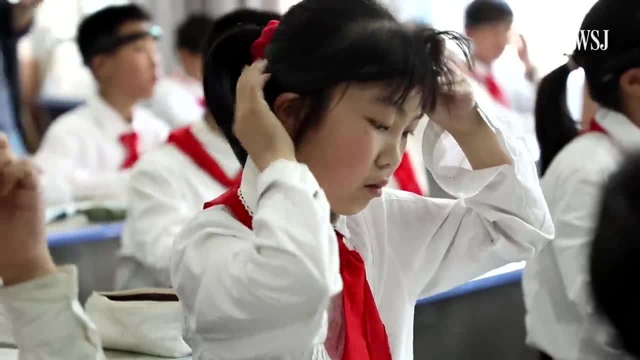 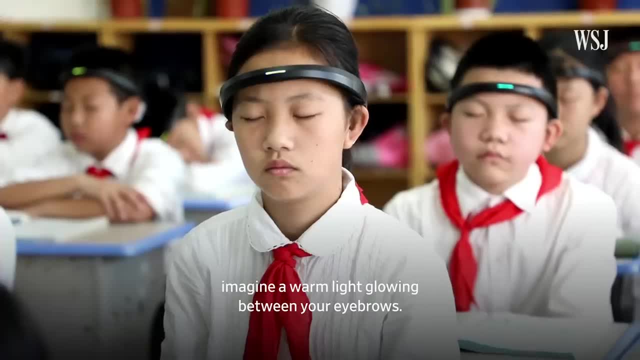 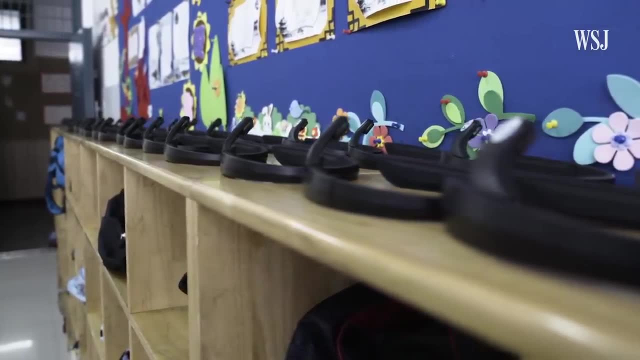 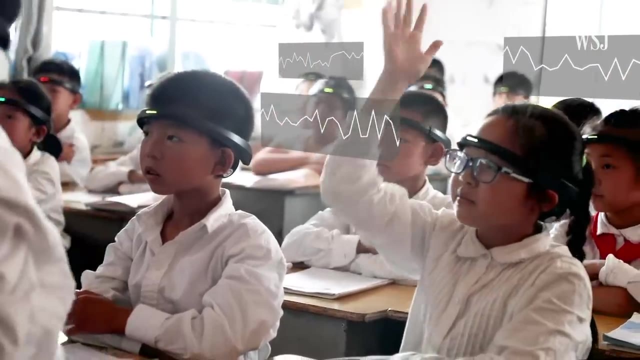 Students then practice meditating. The device is made in China and has three electrodes: two behind the ears and one on the forehead. These sensors pick up electrical signals sent by neurons in the brain. The neural data is then sent in real time to the teacher's computer. 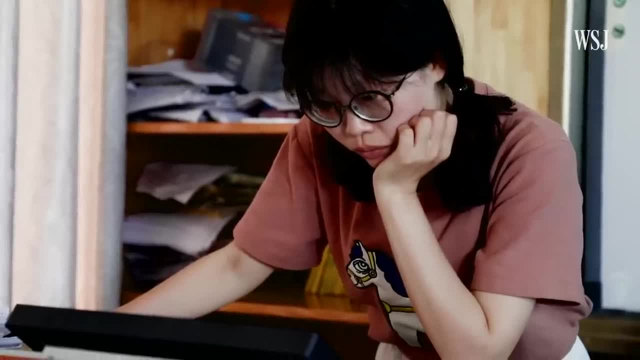 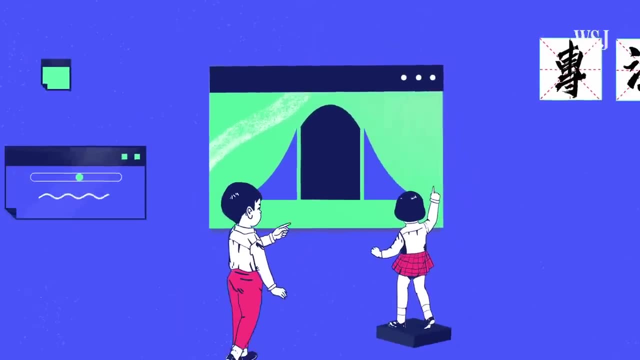 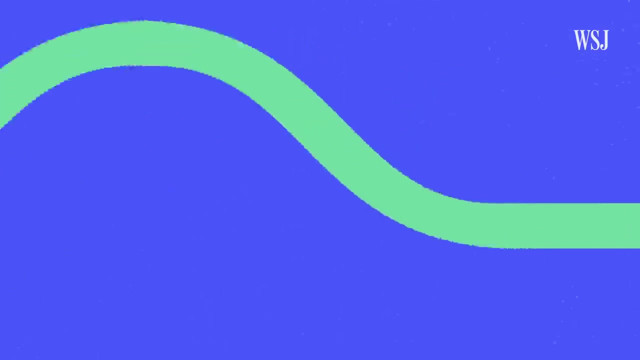 So while students are solving math problems, a teacher can quickly find out who's paying attention and who's not. A report is then generated that shows how well the class was paying attention. It even details each student's concentration level at 10-minute intervals. 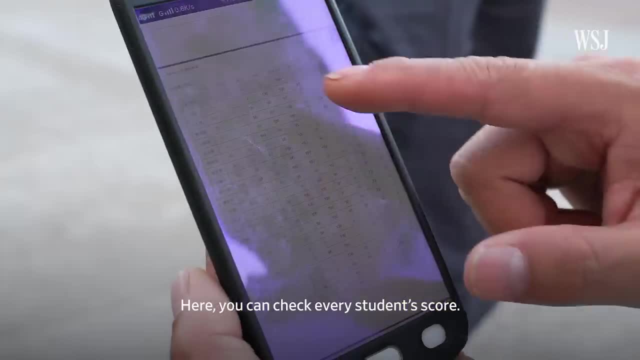 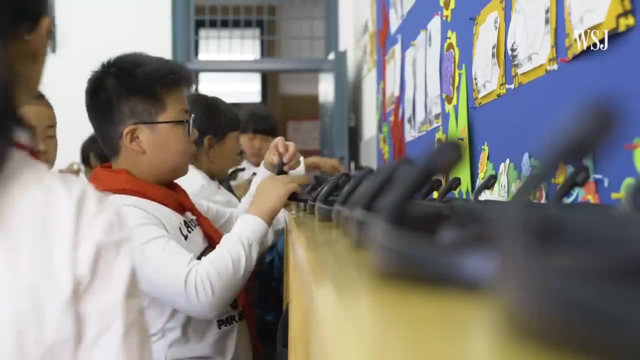 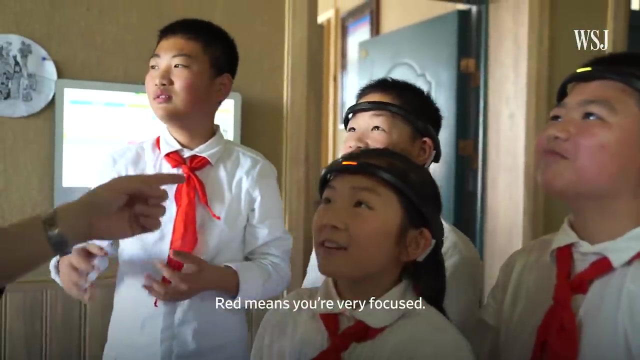 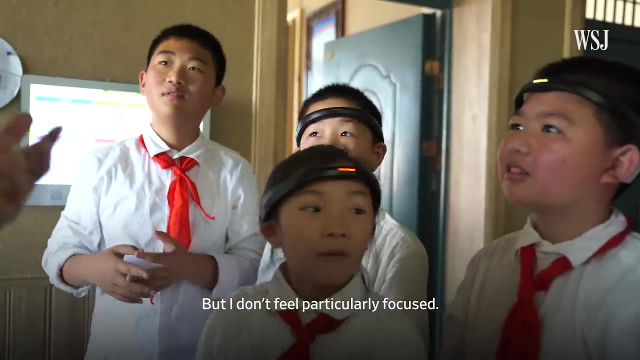 It's then sent to a chat group for parents. The reports are detailed, but whether these devices really work and what they exactly measure isn't as clear. We were curious if the headbands could actually measure concentration, so one of our reporters tried on the device. 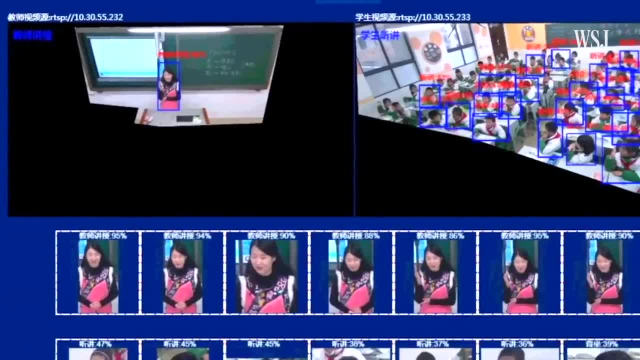 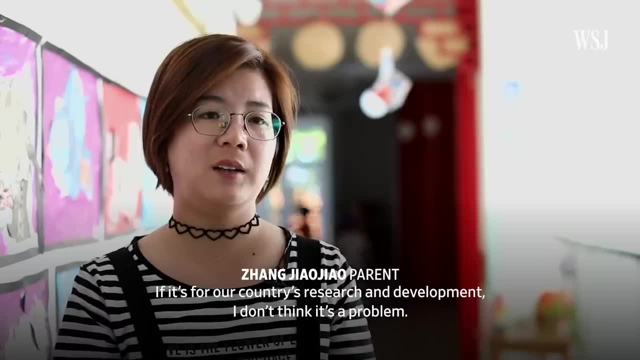 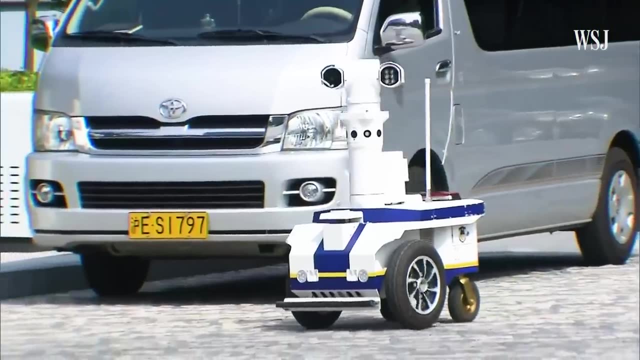 is one of the world's largest experiments in AI education, A program that's supposed to boost students' grades While also feeding powerful algorithms. I think there's nothing wrong with developing it for the sake of the country. The government has poured billions of dollars into the project, bringing together tech giants. 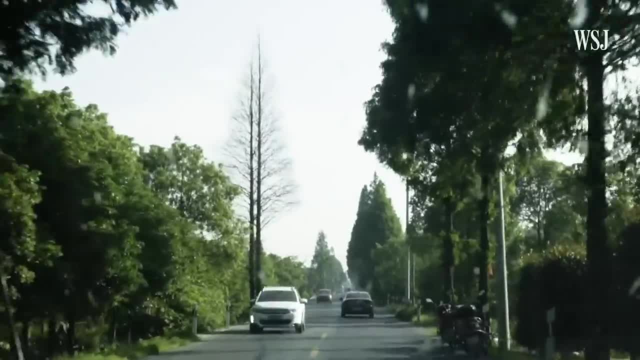 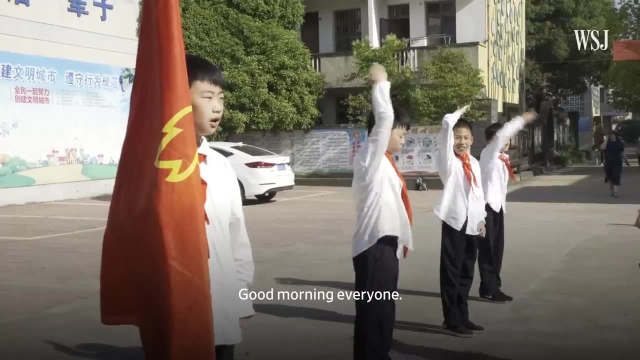 startups and schools. We got exclusive access to a primary school a few hours outside of Shanghai To see first-hand how AI can be used to teach a child at home. The government is also putting a lot of effort into its development. We're going to see if it works. 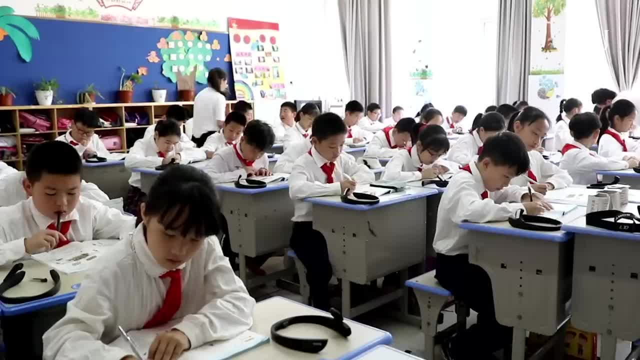 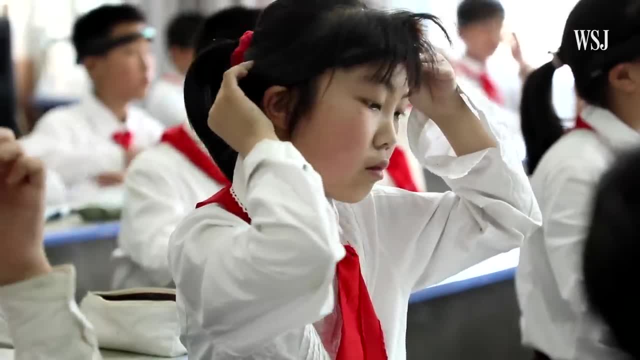 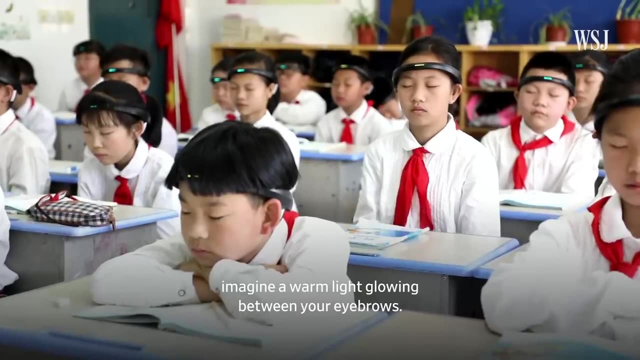 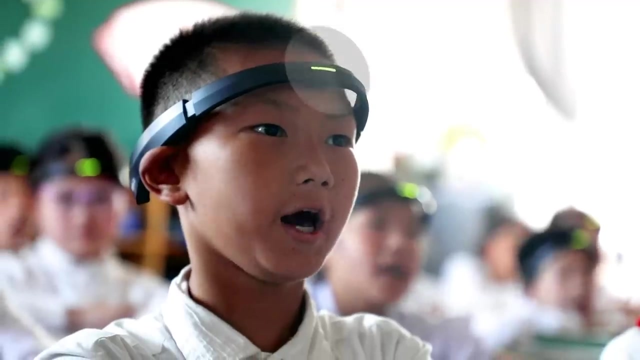 how AI tech is being used in the classroom. For this fifth grade class, the day begins with putting on a brain wave sensing gadget. Students then practice meditating. The device is made in China and has three electrodes: two behind the ears and one on the forehead. 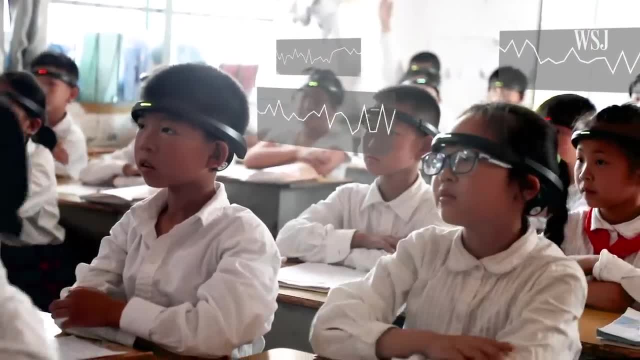 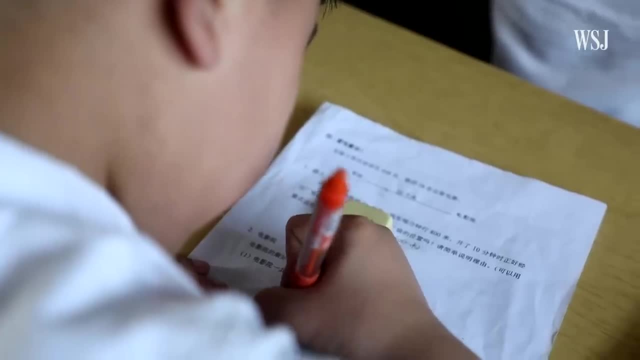 These sensors pick up electrical signals sent by neurons in the brain. The neural data is then sent in real time to the teacher's computer. So while students are solving math problems, a teacher can quickly find out who's paying attention and who's not. 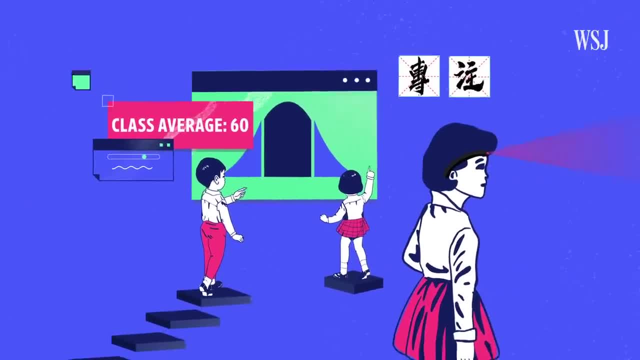 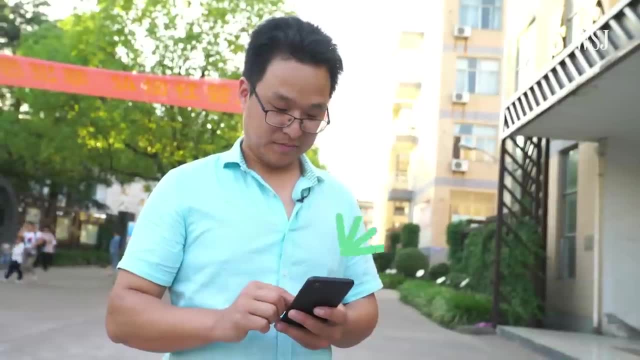 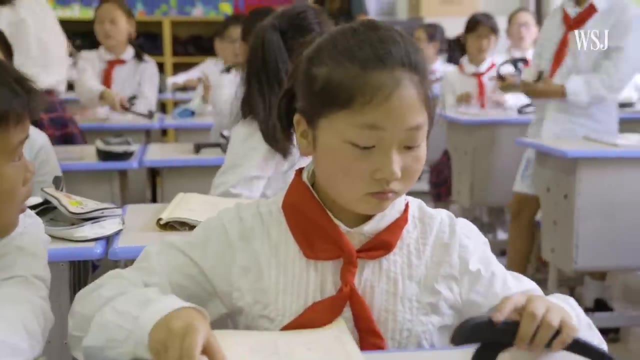 A report is then generated that shows how well the class was paying attention. It even details each student's concentration level at 10-minute intervals. It's then sent to a chat group for parents. The reports are detailed, but whether these devices really work. 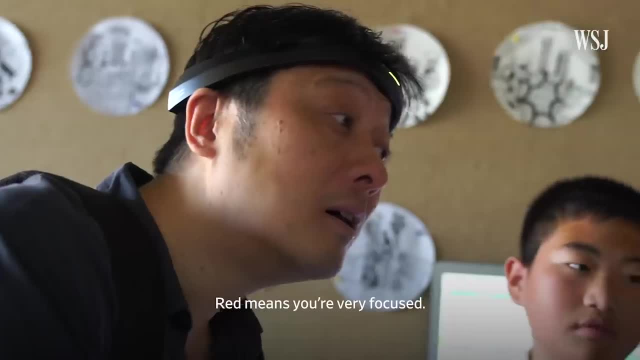 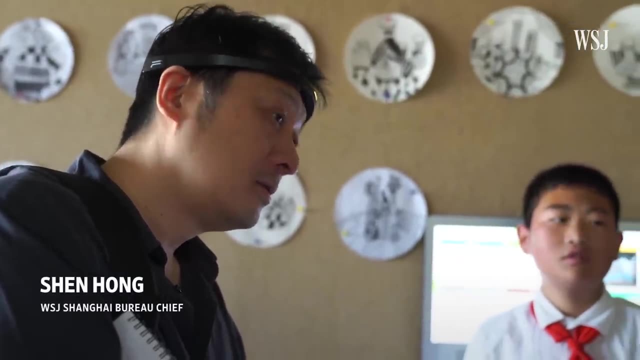 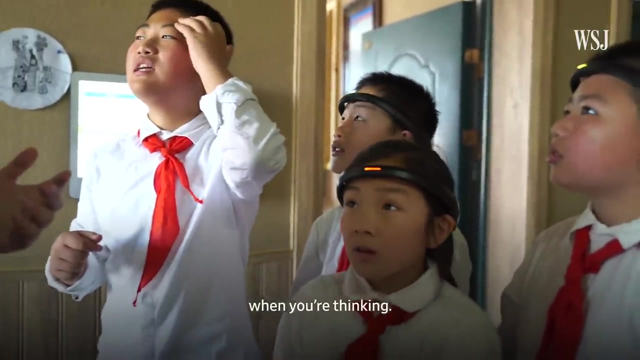 and what they exactly measure isn't as clear. We were curious if the headbands could actually measure concentration, so one of our reporters tried on the device. This is a new technology with still fairly little research, but it's pretty good. This is a new technology with still fairly little research, but it's pretty good. 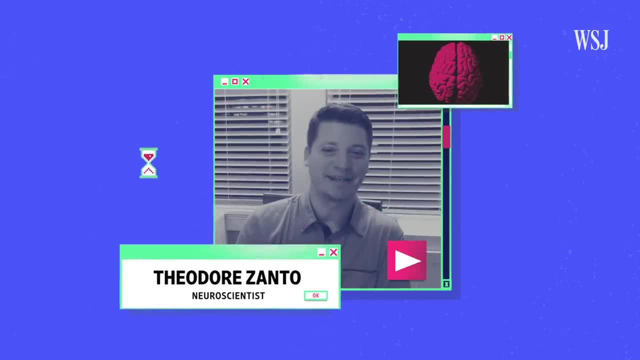 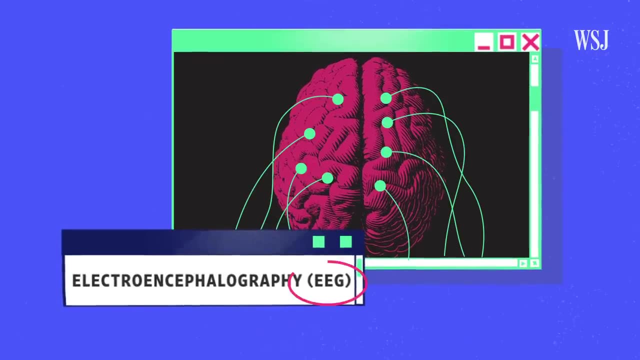 This is a new technology with still fairly little research, but it's pretty good. Theodore Zanto is a neuroscientist at the University of California, San Francisco. He was surprised to learn that this tech called electroencephalography, also known as EEG. 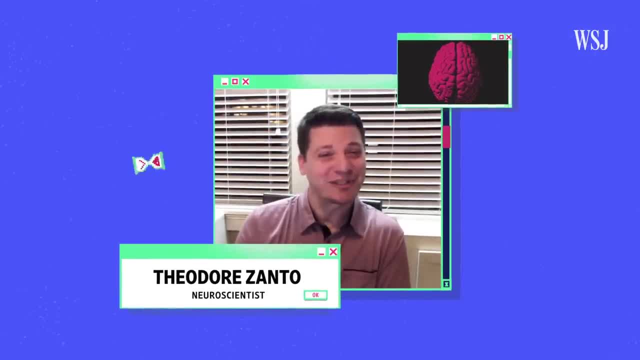 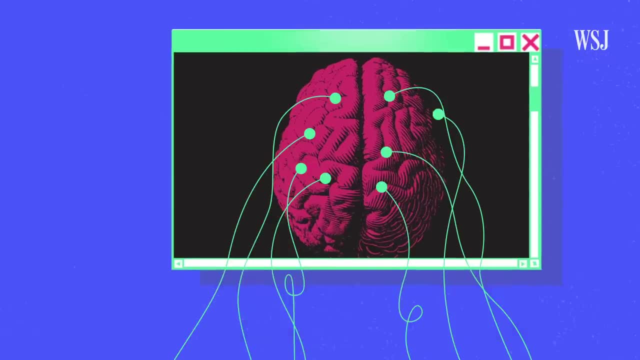 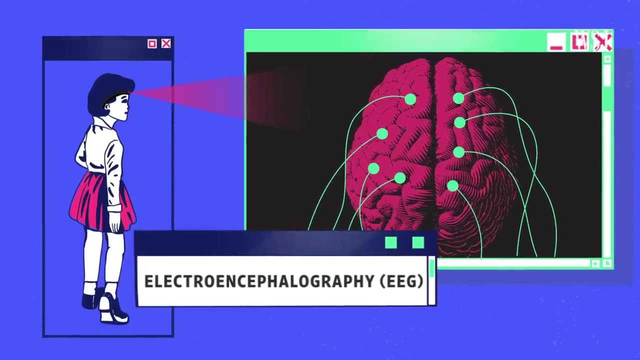 This is a new technology with still fairly little research behind it. Theodore Zanto is a neuroscientist at the University of California. He was surprised to learn that this tech called electroencephalography, also known as EEG, is being used in the classroom on children. 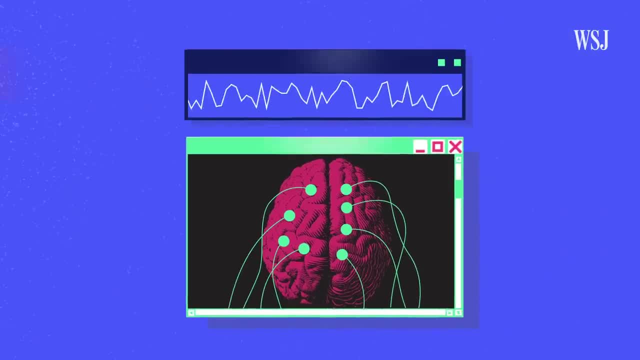 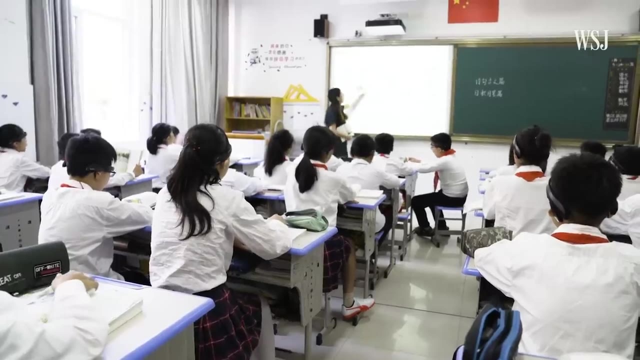 It's usually used by doctors in hospitals and labs. EEG is very susceptible to artifacts, and so if you are itching or just a little fidgety, or the EEG wasn't set up properly so that the electrodes didn't have a good contact, it affects the signal. 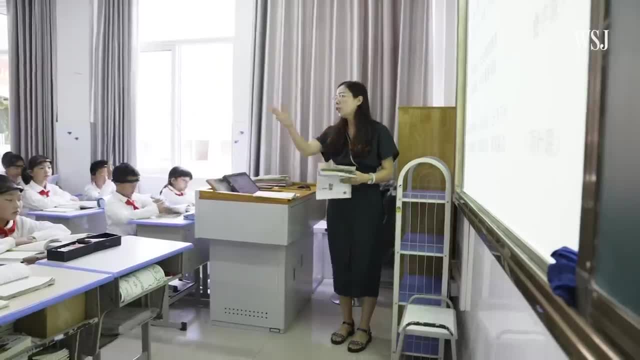 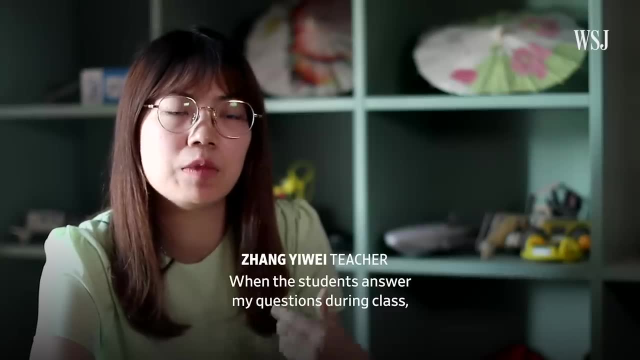 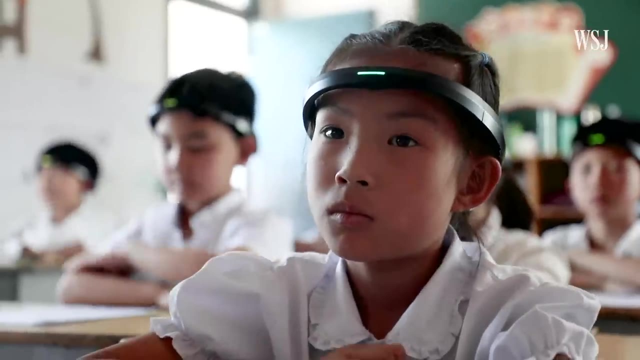 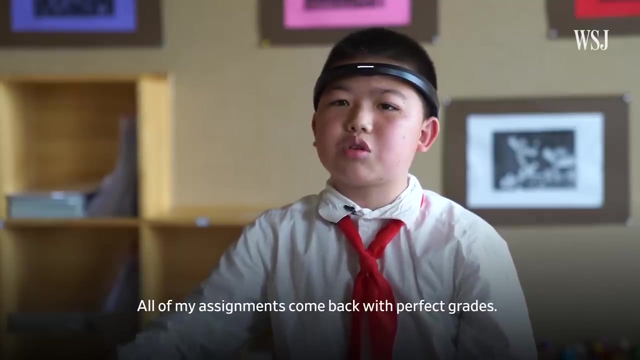 Despite the chances for false readings, the device is still used. Teachers told us the headbands have forced students to become more disciplined. Teachers say the students now pay better attention during class and that has made them study harder and achieve higher scores. But not all students are as enthusiastic. 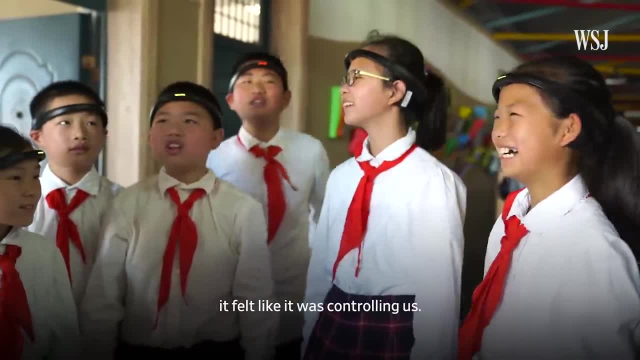 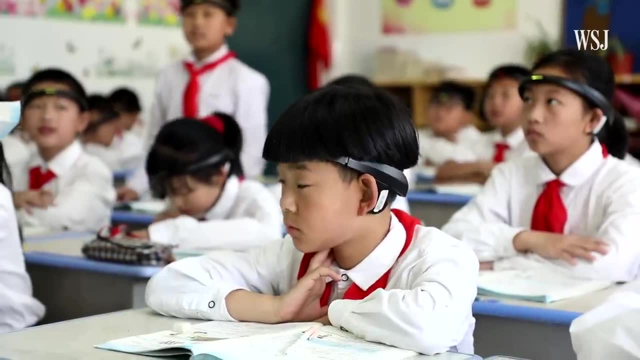 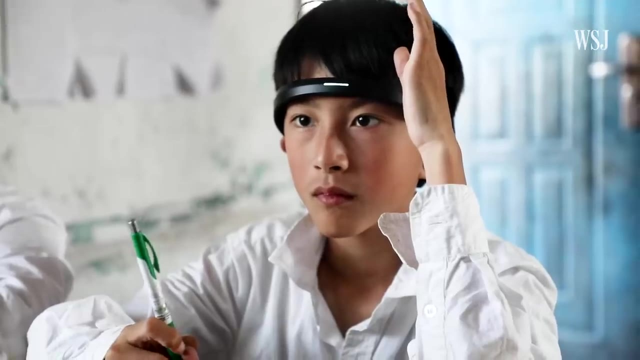 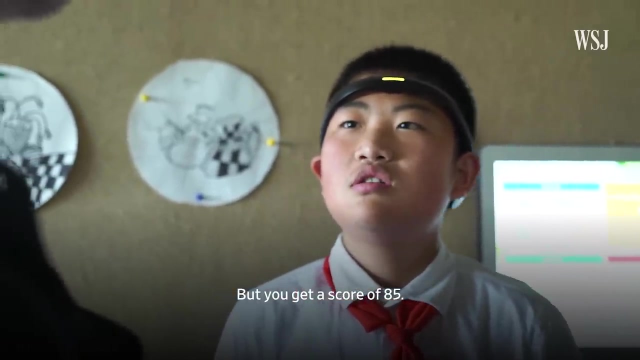 This 5th grader whom we caught dozing off in class told us his parents punished him for low attention scores And that kind of data adds a new kind of pressure for students. If in one exam all the students got 95 points and you got an 85, do you feel like you have? 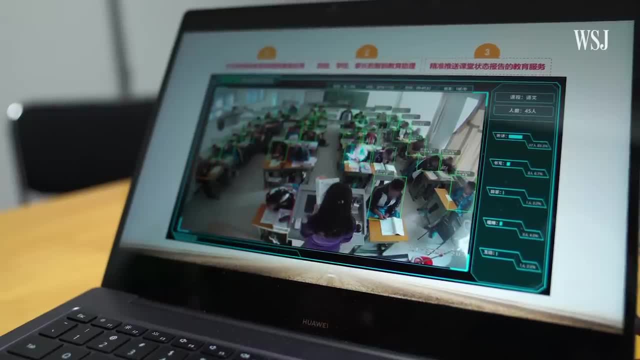 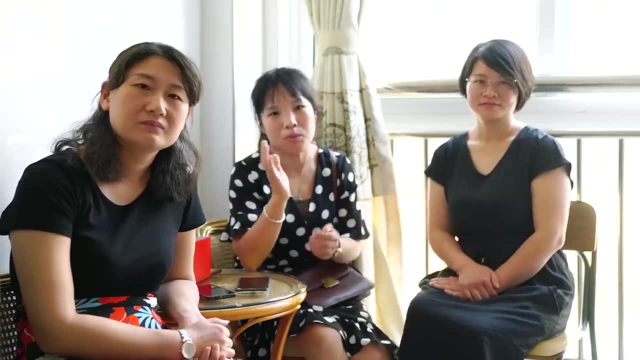 an advantage? No, No. The headmaster's attributes said the data can go to government-funded research projects. We spoke to parents who were unclear about where the data ended up And they didn't seem to care too much. Santos says there's likely no privacy protection at all. 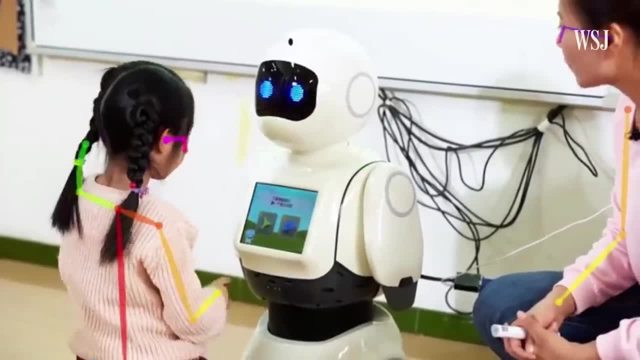 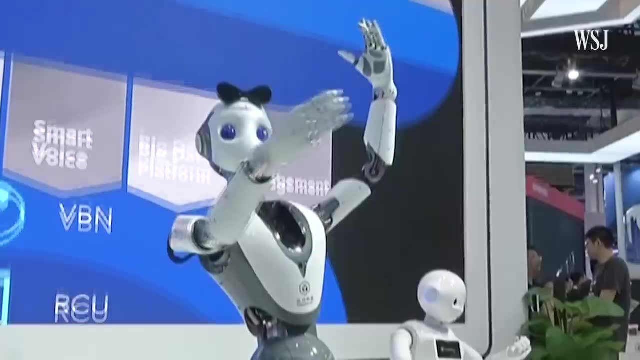 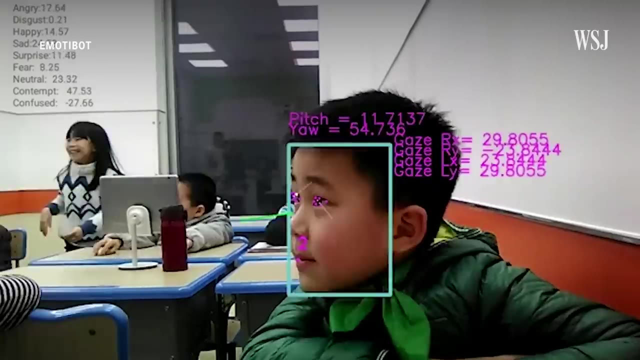 In a classroom. if you're trying to make an assessment of an individual student, you really can't anonymize it. Experts and citizens alike are sounding alarms about various aspects of the country's huge push into artificial intelligence. What These classrooms are? laboratories for future generations. and while these new 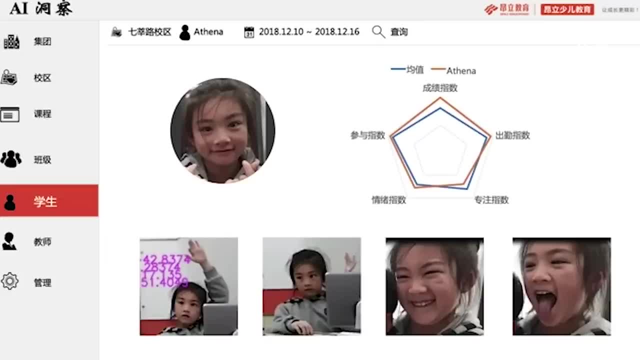 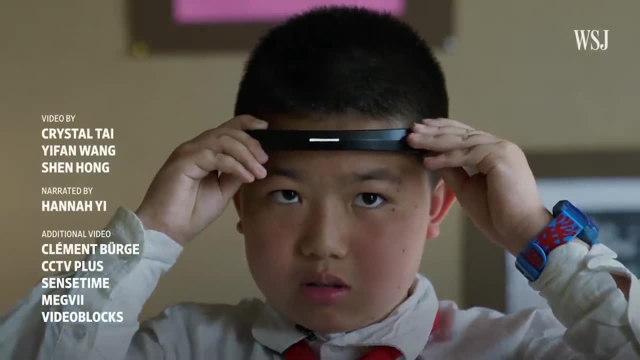 tools may potentially help some 200 million students raise their grades. just how this all works out won't be apparent until they become adult citizens. 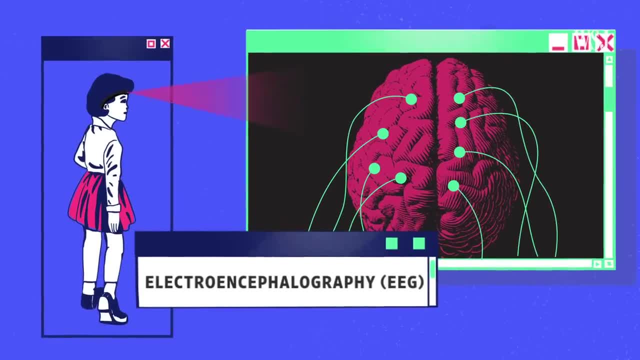 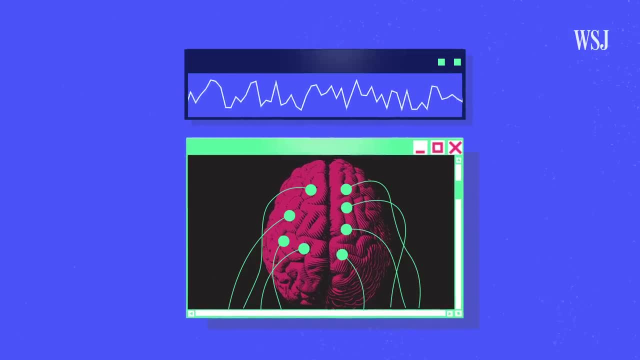 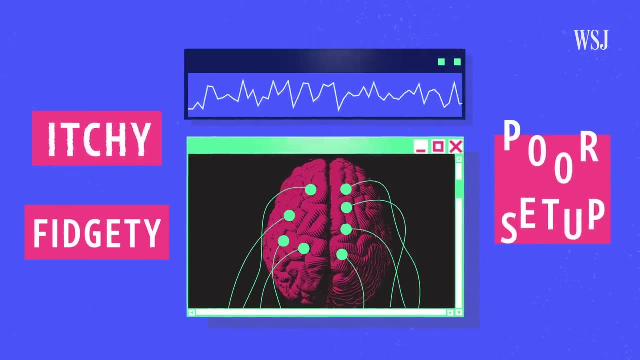 is being used in the classroom on children. It's usually used by doctors in hospitals and labs. EEG is very susceptible to artifacts and so if you are itching or just a little fidgety, or the EEG wasn't set up properly so that the electrodes didn't have a good contact, 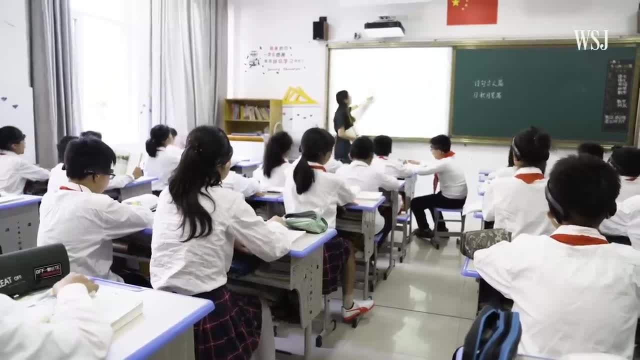 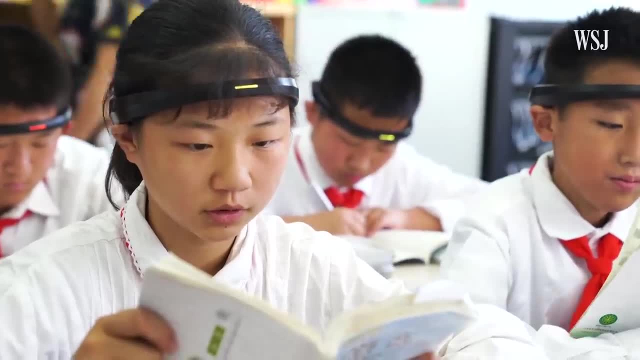 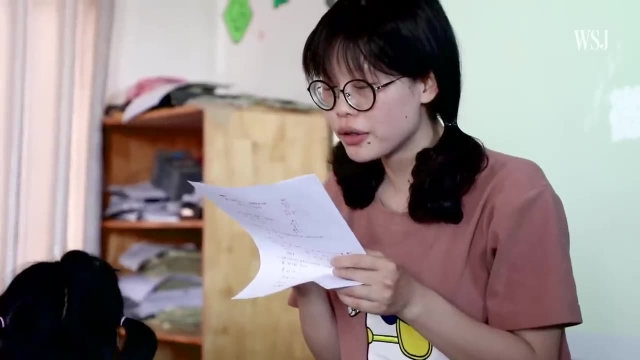 it affects the signal. Despite the chances for false readings, teachers told us the headbands have forced students to become more disciplined. The questions answered in class are louder than usual. Teachers say the students now pay better attention during class and that has made them study harder. 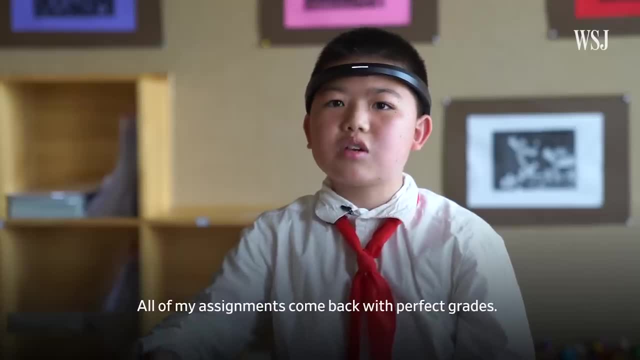 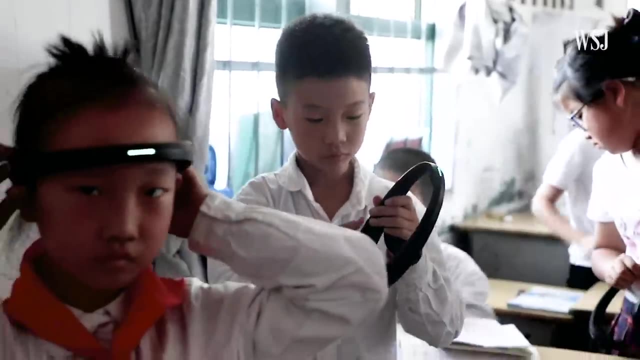 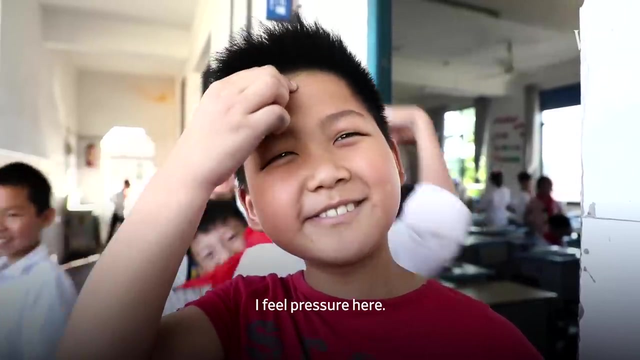 and achieve higher scores In class. I listened carefully. Basically, the homework was done by the whole team, But not all students are as enthusiastic. When I was in elementary school, there was this thought that I felt like I was stuck in a tight spot. 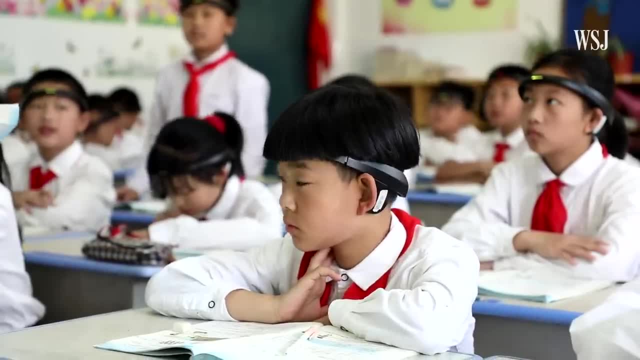 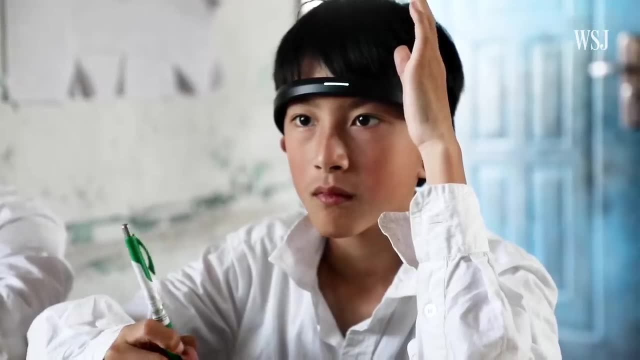 This fifth grader, whom we caught dozing off in class, told us his parents punished him for low attention scores, And that kind of data adds a new kind of pressure for students. Think about it If in one exam all the students got 95 points. 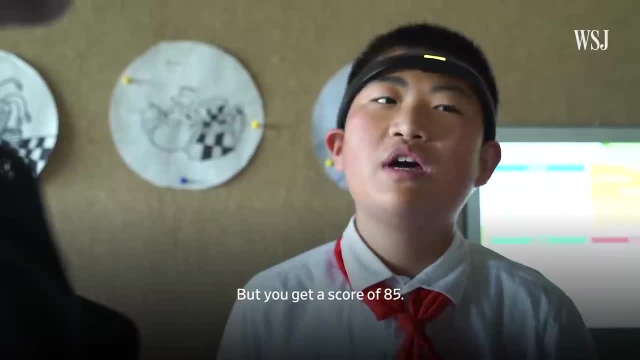 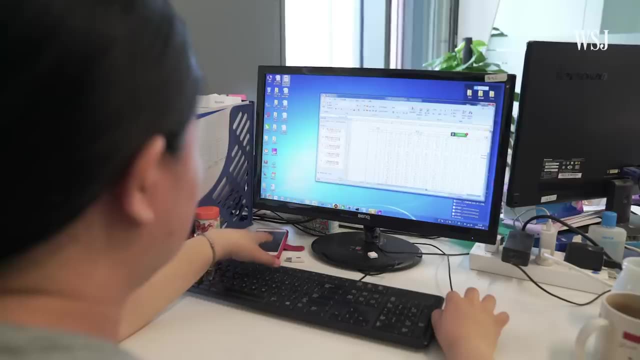 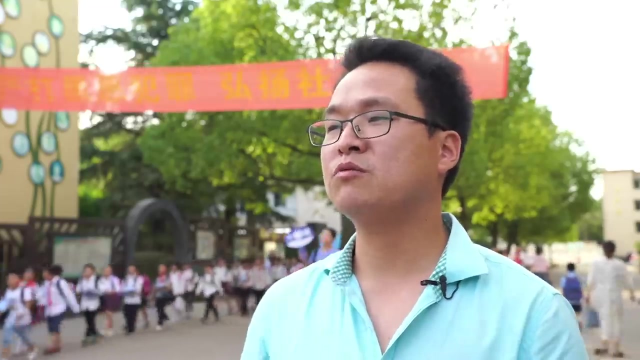 and you got 85 points. Do you feel like you're a little behind? Companies we interviewed said the data can go to government-funded research projects. We spoke to parents who were unclear about where the data ended up and they didn't seem to care too much. 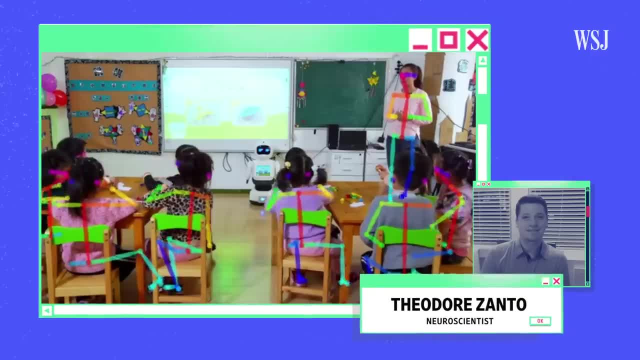 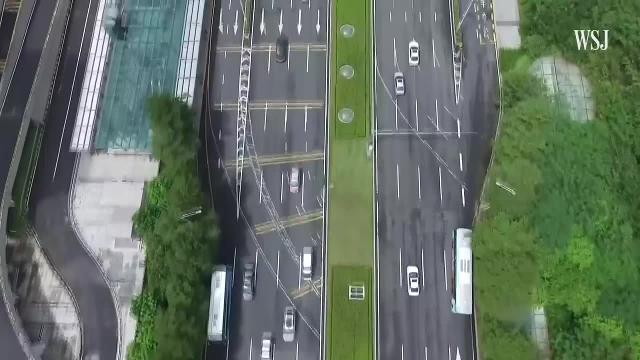 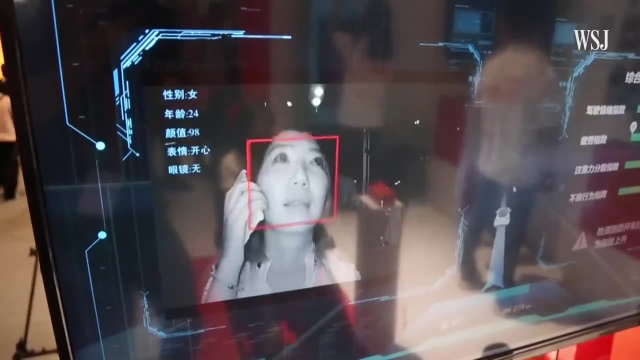 Santos says there's likely no privacy protection at all In a classroom. if you're trying to make an assessment of an individual student, you really can't anonymize it. Experts and citizens alike are sounding alarms about various aspects of the country's huge push into artificial intelligence. 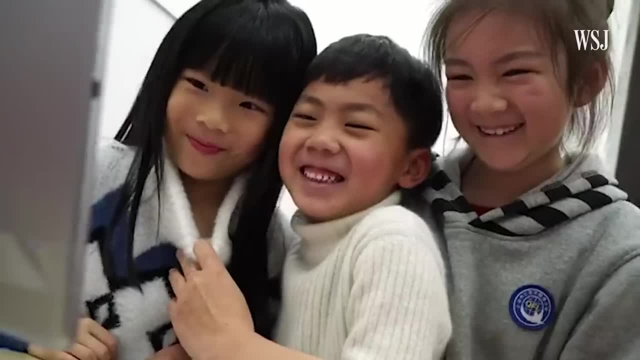 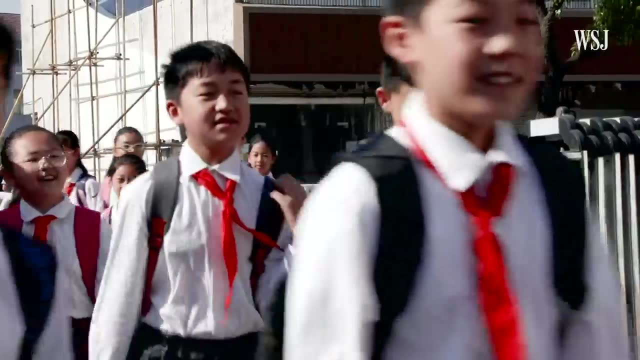 These classrooms are laboratories for future generations, And while these new tools may potentially help some 200 million students raise their grades, just how this all works out won't be apparent until they become adult citizens.